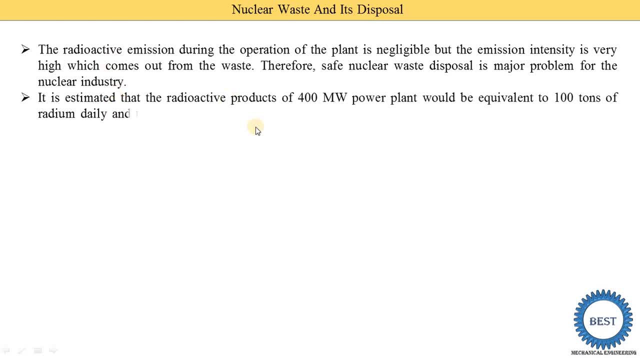 So it is estimate that radioactive product of 400 megawatt power plant will be equivalent to 100 tons of radium daily, And the radioactive effect of this plant product, if we expose to the atmosphere, will kill all the living organisms within the area of about 160 square kilometers. 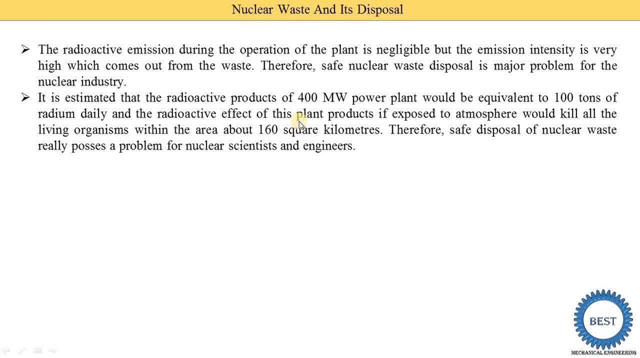 They kill the adult animals or birds or even the agriculture products Around the 160 square kilometers, So this is a very large area. Therefore, safe disposal of nuclear waste really causes a problems for the nuclear scientists and engineers. The waste produced in the nuclear power plant may be in the three form: 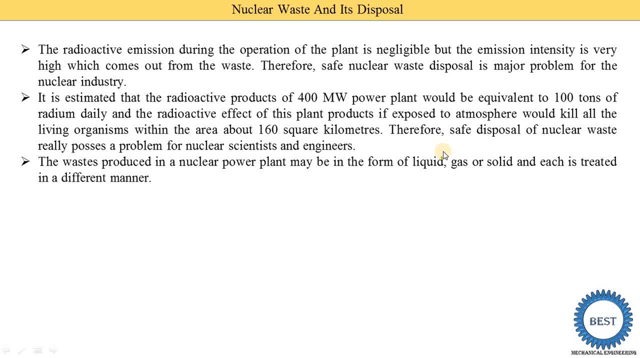 It may be liquid, gas or a solid, And each is treated in a different matters Means the liquid waste is dispose as a some other matters. For the gas or a solid, the disposal matters are different. So now we understand in the detail how the solid gas and liquid waste are treated. 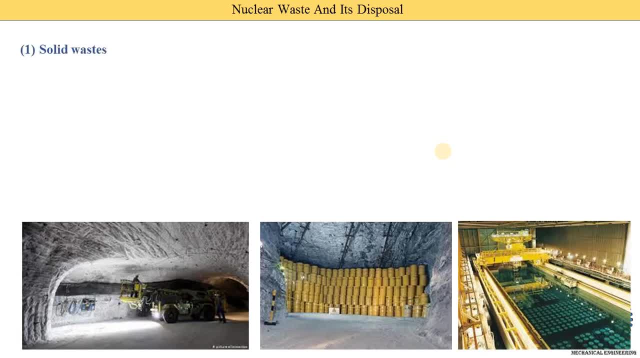 So first we understand about the solid waste. Means the nuclear waste are present in the solid state. So there is a different way to disposals of a solid waste. Solid radioactive waste will arise from the use of filter Sludge from the cooling ponds. 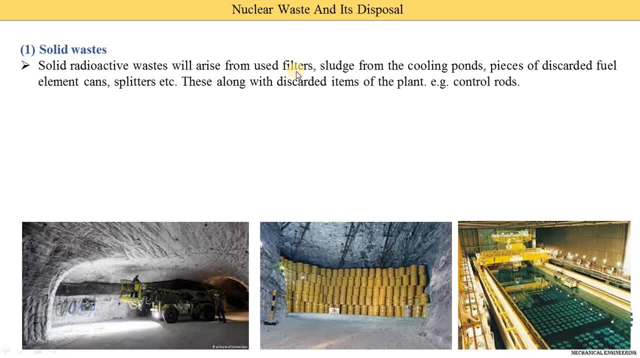 Means we are use the various filters in the nuclear power plants. So when we change these filters, So these filters are nuclear waste for us. Sludge from the cooling ponds Piece of discarded fuel element cans and the splitters Means the fuel coming out from the nuclear plant. it is also a waste. 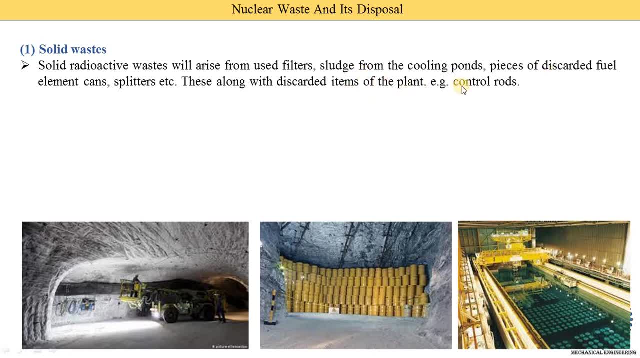 These, along with discarded items of the plant, like as the control role, means some component we need to replace After some times. this is also consider as the solid waste, like as the control roles. So these are the various source of the solid waste. So there are many way for disposing of the solid fission products. 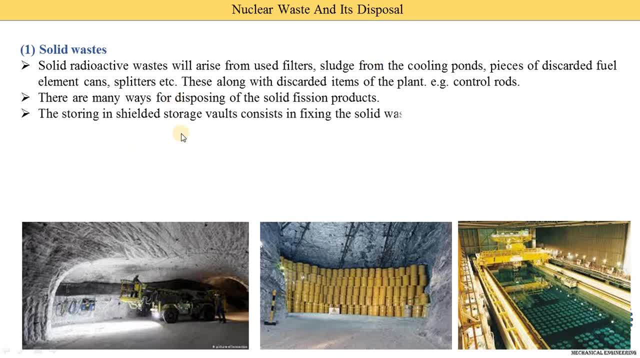 So first matters are the storing in a shielding storage wallets consist in fixing the solid waste in a borosilicate glass- Means all the solid waste coming Is stored in a borosilicate glass- And then storing this glass in a leak tight capsule. 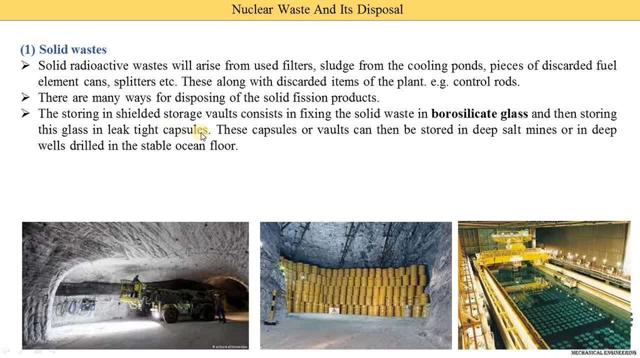 Means, first the solid waste is stored in a borosilicate glass And then, after this borosilicate glass is put in the liquid, tight capsules, And then, after these capsules or wallets can be stored in a deep salt mines or in a deep, well drilled in the stable ocean floors. 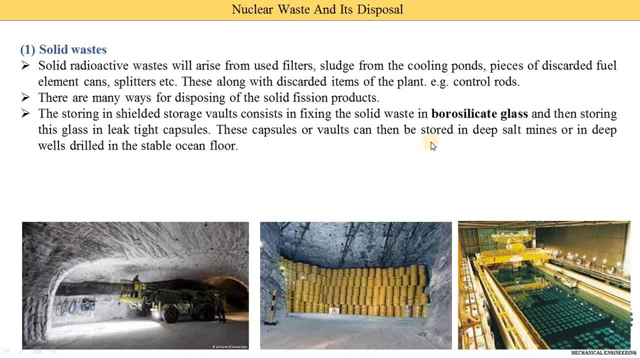 Means these capsules are putted in a salt mines Or either they are put in a deep well drilled in a stable ocean floor. Means we drill the one hole in a ocean floors And then this capsule is supplied. But oceans are required to the stable oceans. 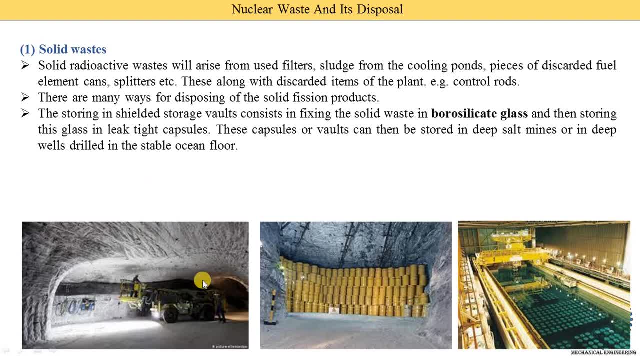 So here you see in this various image. So here these cans are stored in a salt mines. This is also salt mines. Sometimes they are stored in the water levels And then, after they are discard to some other places, The combustible solid waste is burn in a incinerators. 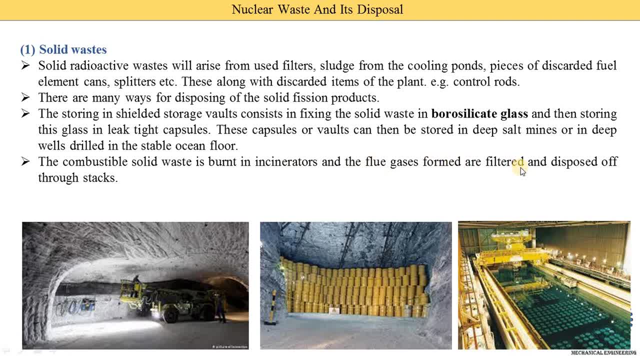 And then flue gases forms are filters And dispose of through stacks, Means. some of the solid waste are combustible, So it is combustion of the solid waste is carried out And this combustion, flue gases, are passed from the some filters And then from the filters. 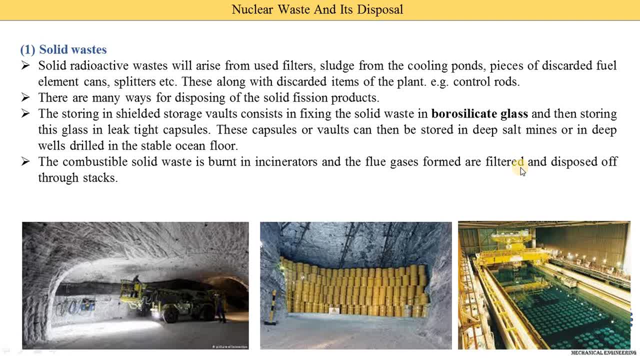 The further flue gases are supplied to the atmospheres. Active solid waste are stored in a water for about 100 or more days To allow the radioactivity to decay- Means some waste are active. So first we need to decay this radioactivity. 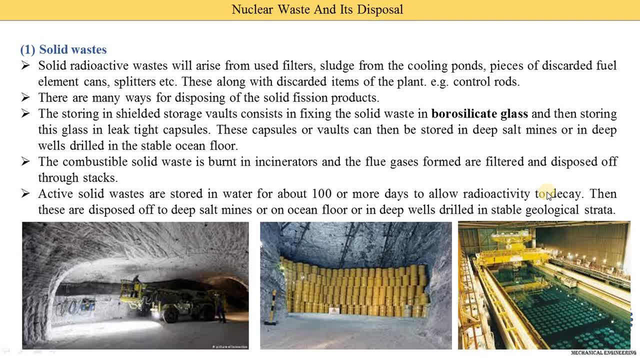 By storing the solid waste in a water for a 100 days. So in this last image you see The solid waste are stored in a water for the 100 days. Then these are dispose of to deep salt mines Or on a ocean floor. 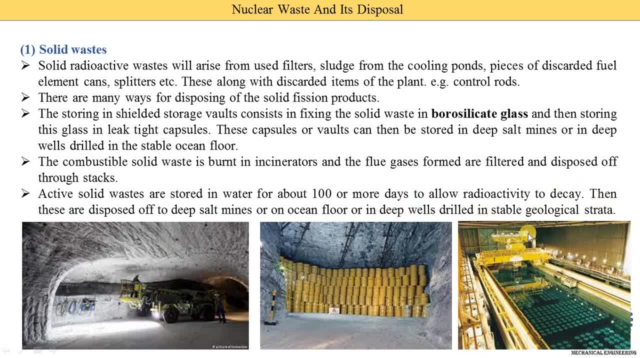 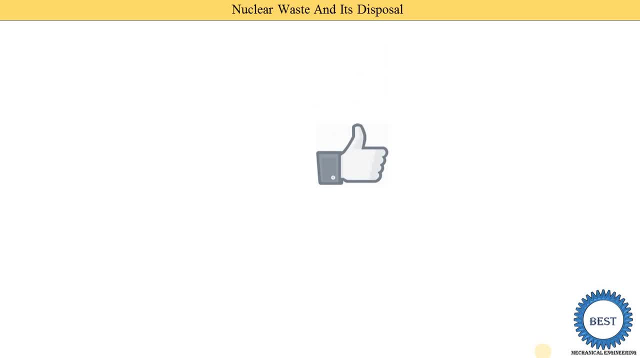 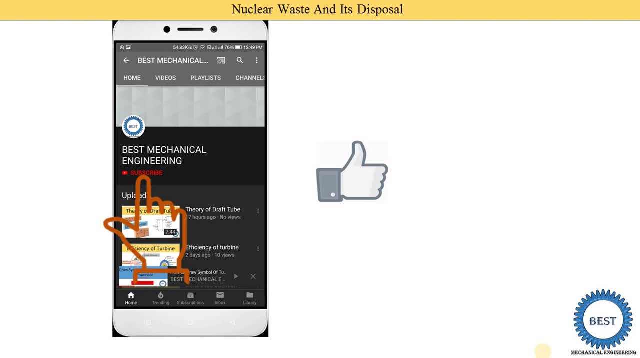 Or in a deep well drilled in a stable geological strata. So these are the what is the solid waste And how the solid waste are dispose. Now, before moving ahead, I request to like the video And subscribe my channel For watching the more video related to power plant engineering. 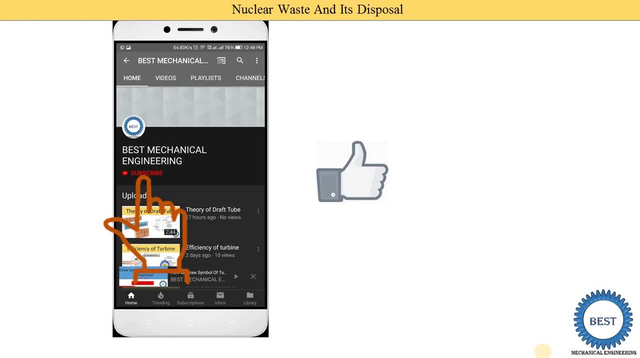 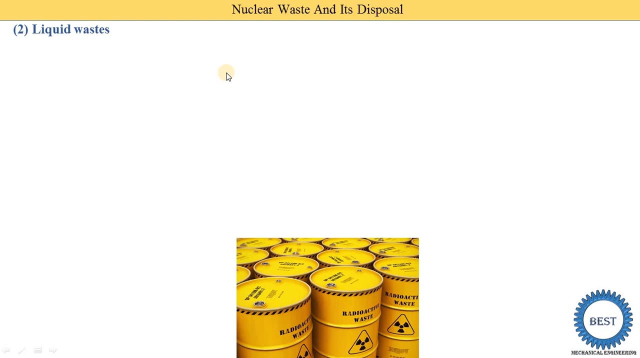 Or other subject of this Mechanical engineering. For power plant engineering, Various link is provide in descriptions As well as in a car. for other subject, I request to visit the playlist. Now we understand What is the liquid waste And how these liquid waste are dispose. 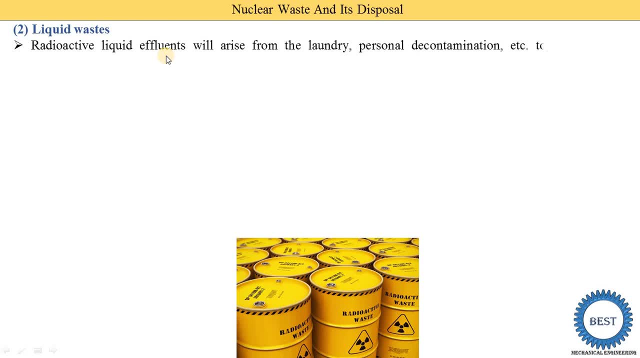 Radioactive liquid effluents will arise from the laundry Personal decontamination. It's together with activity Accumulating from the corrosions of the irradiated fuel elements In a storage ponds Means. some fuels are store In a storage ponds. 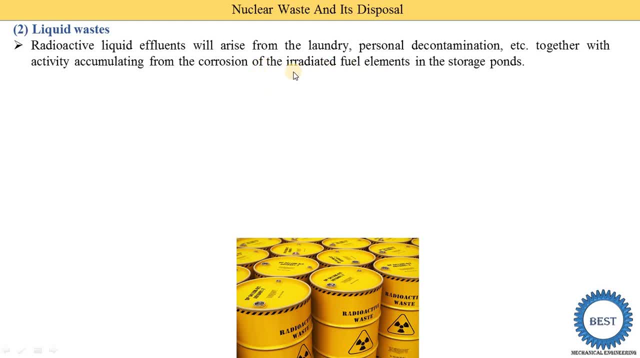 At that times The liquid waste are coming From the laundry And for the personal decontamination The liquid waste are coming. The disposal of liquid waste Is done in a two way. First one is the dilutions. Dilution means: 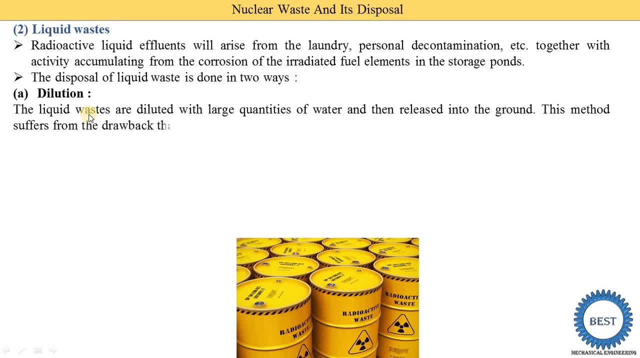 The liquid waste are mix with the water Means its intensity, are dilute. The liquid waste are diluted With a large quantity of water. So these waste are mix with the large quantity of water Means, the its intensities are reduced And then release into the ground. 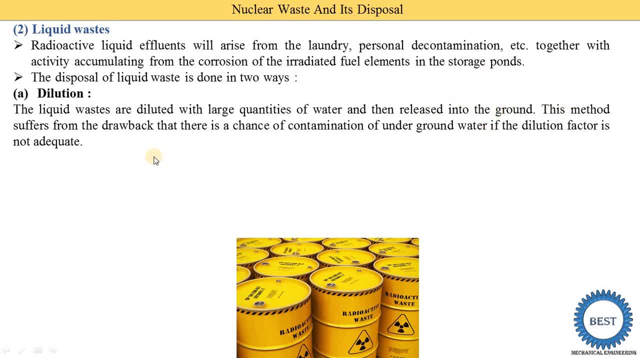 So these matters suffer from the drawback that There is a chances of contamination of underground water If the dilution factor is not admincant, Means if we are not provide sufficient Quantity of water for the dilutions, At that time the dilution factor is not admincant. 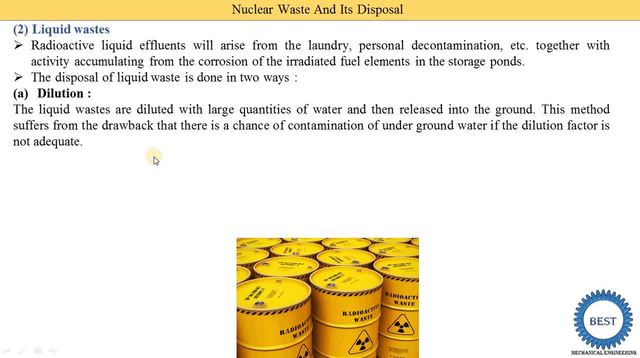 Means dilution factor is less. At that time there is a chances is that The underground water is also contaminated With the radioactive material. So it is the harmful for the human persons Or for our environments. Second matter is the concentration to small volumes. 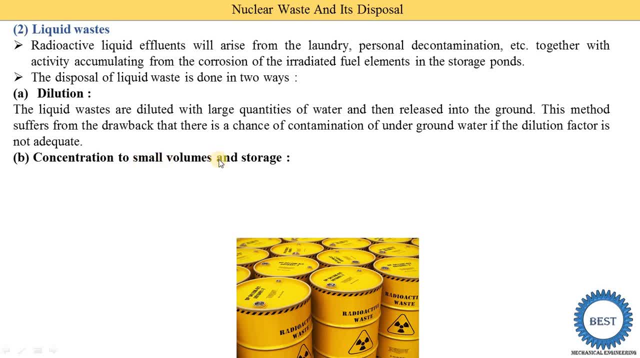 And the storage Means. the liquid waste is store In a some volumes Or a some vessels, And then this vessels are store When this dilutions of radioactive liquid waste Is not desirable Due to amount of nature of isotopes Means, due to same reasons. 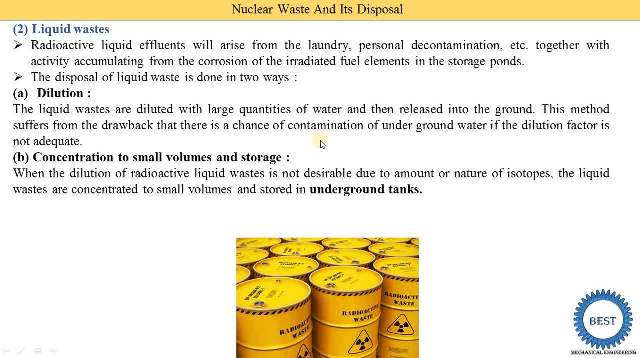 The dilution is not possible. Then what happen? The liquid waste are concentrated To small volume And store in underground tanks, And the tank should be of Unsure long term strength And the leakage of liquid from the tank Should not be takes place. 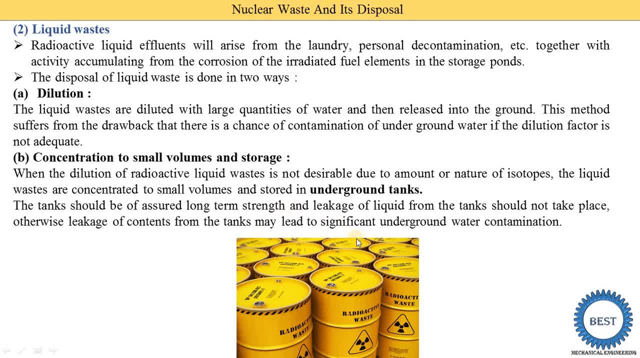 Otherwise, leakage of contents From the tank may be Lead to significant underground water contamination Means. when we store the liquid waste In a some tank Or a some vessels, At that time we need to check its long term strength. Leakage is not possible from the tank. 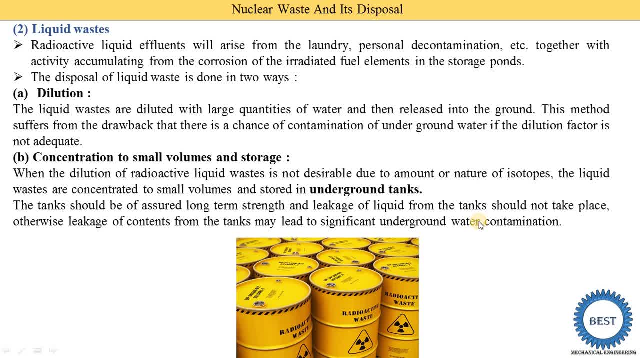 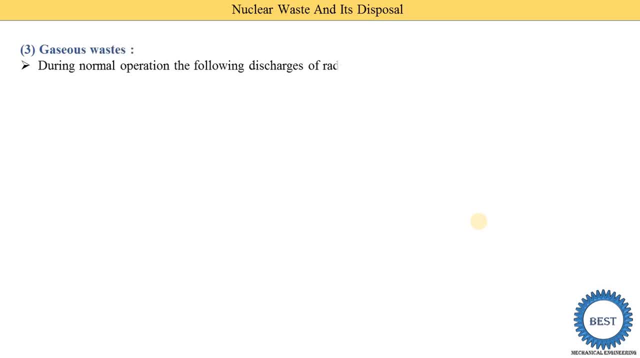 Because some leakage is carried out from the tank, Then they creates the problems Now. the third waste is the Gaseous waste. During the normal operation The following discharge of radioactive Gases, coolant will occurs, So leakage from the pressure circuit. 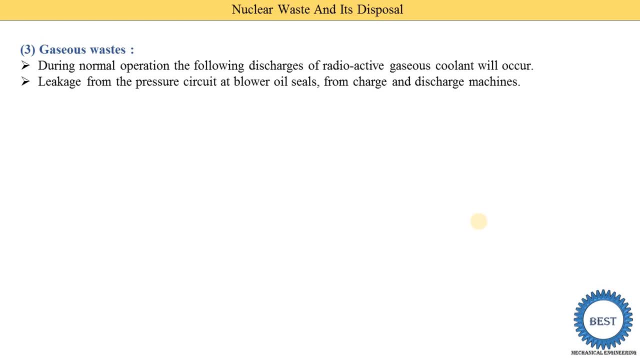 At the blower oil seals From the charge and discharge machines, So crepton and Ionite gas Coming out from the spent nuclear fuels Means from the nuclear fuels The crepton and ionite gases Coming out, And these gases are radioactive. 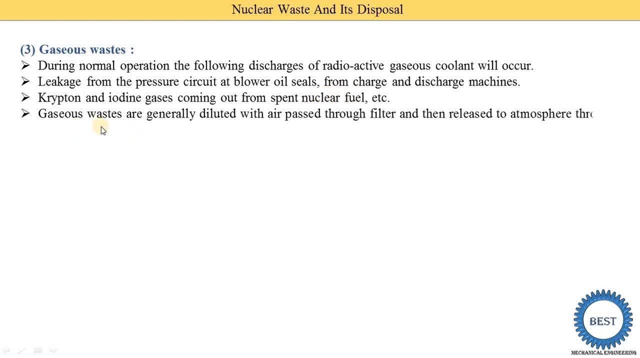 Because they are coming out From these nuclear fuels. Gaseous waste Are generally diluted With air, Passed through filters And then released to atmospheres Through the filters And then released to atmosphere Through large chimney Means gaseous waste coming out. 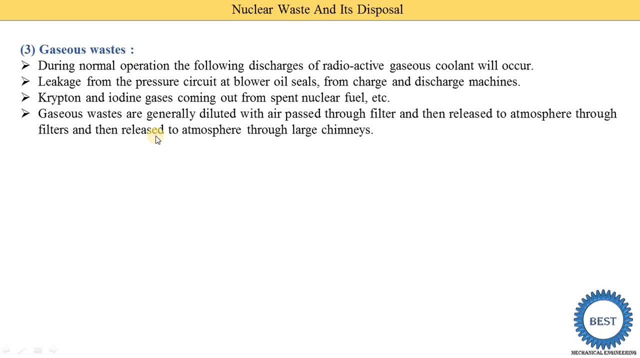 From the plant Are diluted with the air Passed through the filters. Means this Diluted gases are passed from the filters Or they are mixed with the Large quantity of the airs And then, after they are released To the filter. 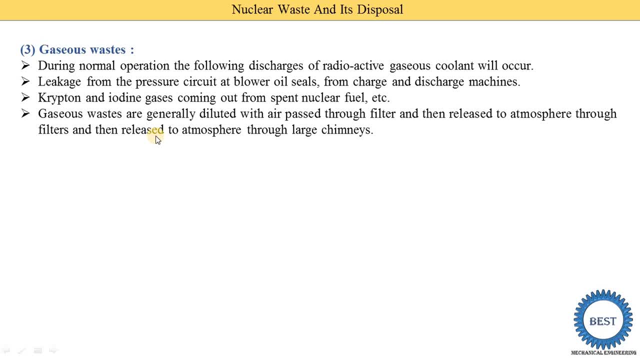 Means they are passed from the filters And from these filters They are supplied to the atmosphere By chimney. Crepton is removed By cryogenic treatment Of dissolved gas streams And packed in a gas cylinder Under a pressure, Means crepton and ionite gases. 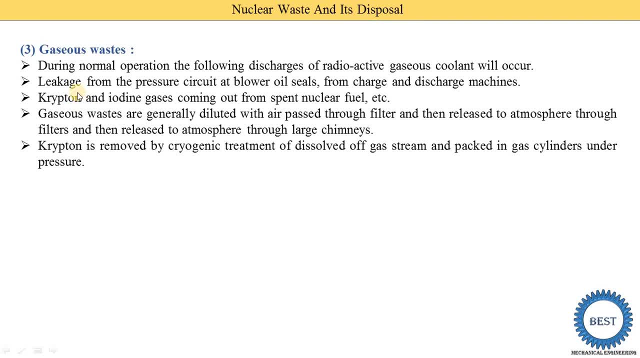 So methods are different For the disposal Means. creptons are disposed by some other way, Ionite is disposed by some other way. So crepton is Removed by cryogenic treatment Of the dissolved gas stream And then after This dissolved process,